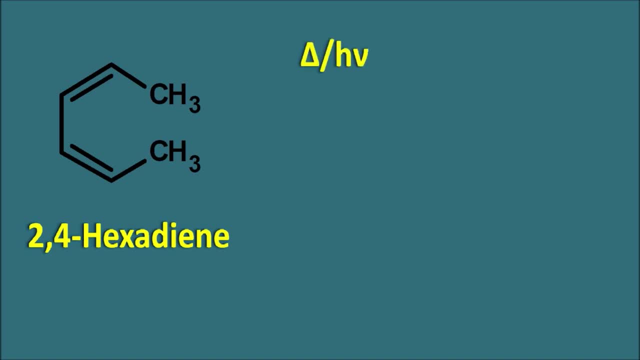 which is having the two double bonds. and when we supply the energy in the form of either photo or thermal energy, this compound can undergo the electrocyclic reaction. So here, this pi bond is going to be converted into a sigma bond, and this pi bond is going to be delocalized such that it is 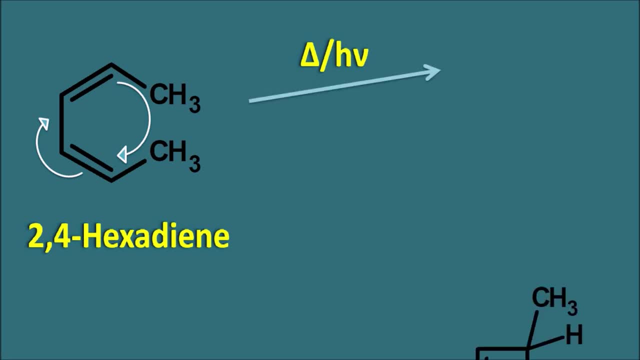 going to give a cyclic product, and this cyclic product may be like this or it may be like this. Here you can see that both structures are having the similar connectivity, but the methyl groups are arranged in different way. The first one- the methyl groups are on the same side, so this is the 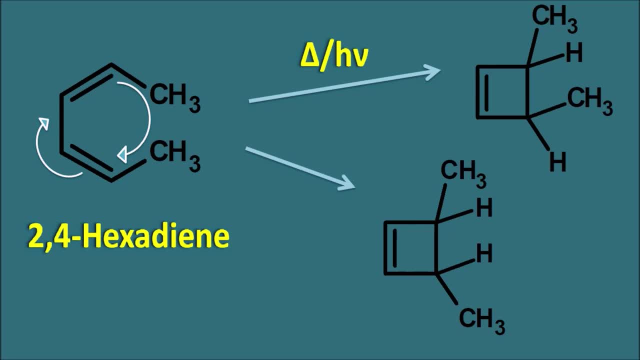 cis isomer, and in the second one the methyl groups are on the opposite side, so it is a trans isomer. So how can we know whether this reaction produces cis isomer or trans isomer? It is very easy to know. Let us see how it works. 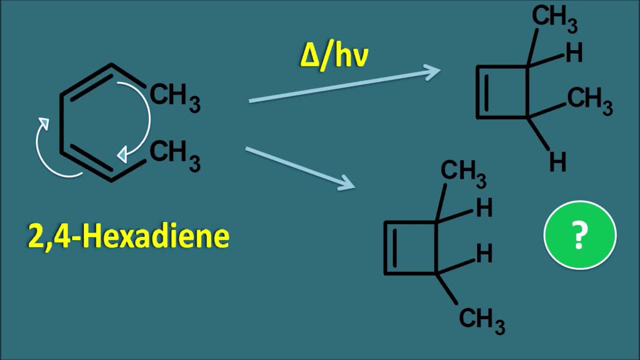 The configuration of the product depends on the configuration of the reactant, as well as which type of source we are going to use, whether the thermal source or photo source. Based on that, we can fix the configuration of the product Today, in this video, we will see one of the easy. 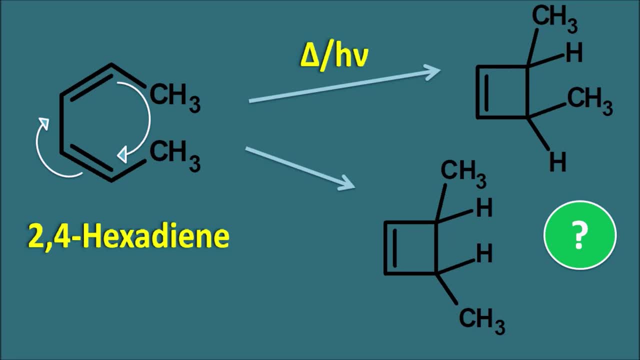 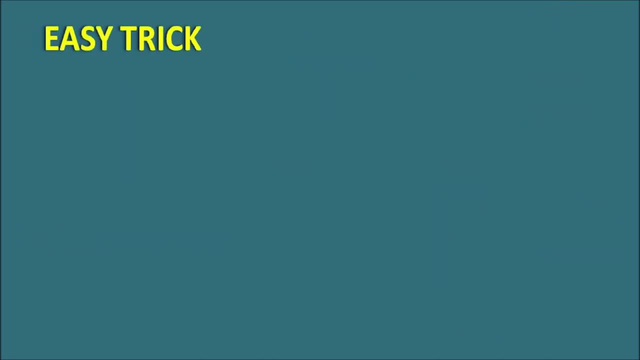 trick. in order to assess what is the configuration of the product, based on the configuration of the reactant and the type of source we are going to use Here, we have to simply remember E, T, C. What about the? E? and T indicates E indicates even and T indicates the. 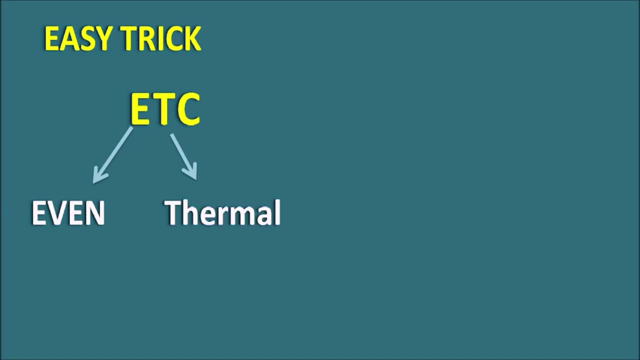 thermal. So even number of pi bonds are there in the reactant and we are going to use the source as a thermal energy, Then the product will have the configuration which is indicated by letter C. So C indicates it is the cis isomer. So here we can remember even and thermal combination. 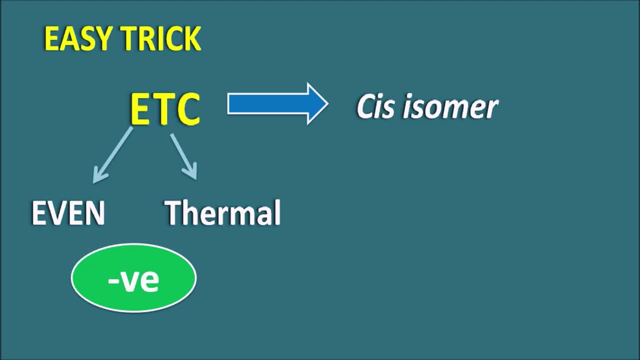 has negative value and when this is negative, it gives the cis isomer. and any of this condition is going to be changed. it gives the opposite isomer, that is, the trans isomer, For example, in place of even number of pi bonds, if the reactant is having the odd number of pi bonds. 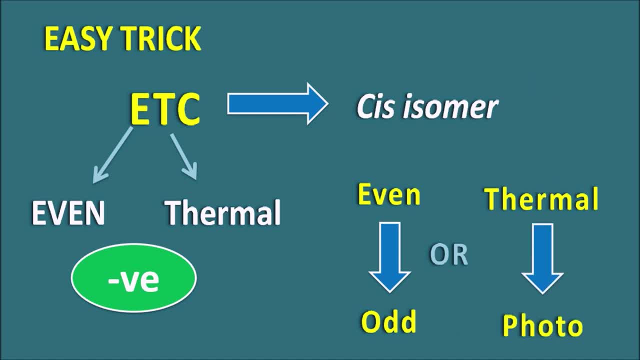 otherwise, instead of the thermal energy we are going to use the photo energy. then it gives the opposite isomer, that means the trans isomer. So any of this condition is going to be changed, the configuration will be reversed. and here, if two conditions are going to be changed, again it gives. 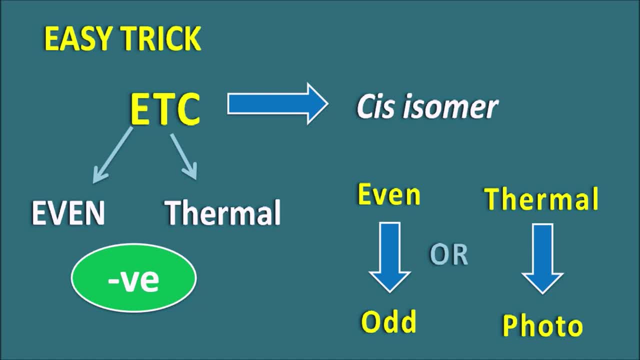 the same isomer. In this way, we can use this easy trick. but in order to understand this easy trick, first of all let us see the different types of configuration that can be observed with the electrocyclic reactions and then we will see the configuration of the product based on the configuration. 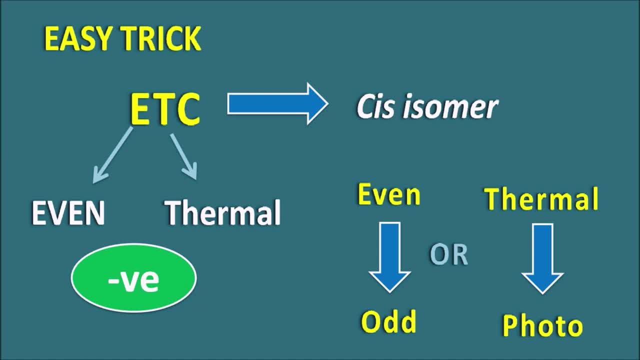 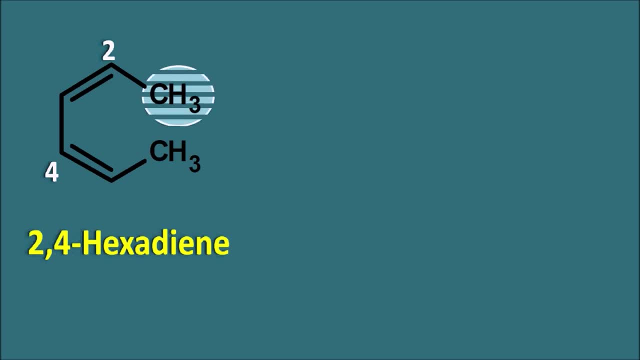 And then we will apply this trick to guess the right configuration of the product. Now already we have seen the 2,4 hexadiene. so this is the second carbon and this is the fourth carbon. and here the first double bond is attached with one methyl group. similarly, second double bond is: 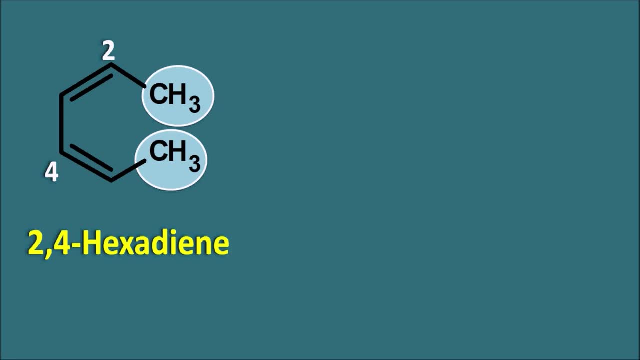 attached with the another methyl group, Based on the orientation of this methyl group. now this 2,4 hexadiene can exist as different types of isomers. For example, this is one of the isomer and here you can see, here the methyl group is opposite side to the double bond. that means it is having 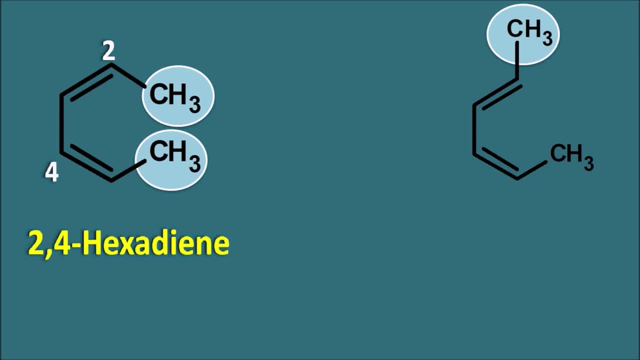 opposite configuration, which we can indicate by the letter e. similarly, if you see the methyl group here, it is on the same side of the double bond, which we can indicate by the letter z. so according to the e and z nomenclature now this molecule can be represented with the configuration 2e4z. 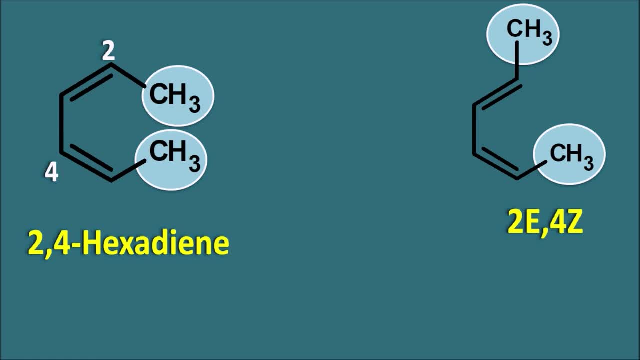 at the second position, e configuration. at the fourth position, z configuration. similarly, we can write the another configuration where the both of these methyl groups are opposite to the double bond, and then we can write the second configuration. in this way we can write the different types of configurations. so here we have represented the two configurations. now let us take the 2e4z. 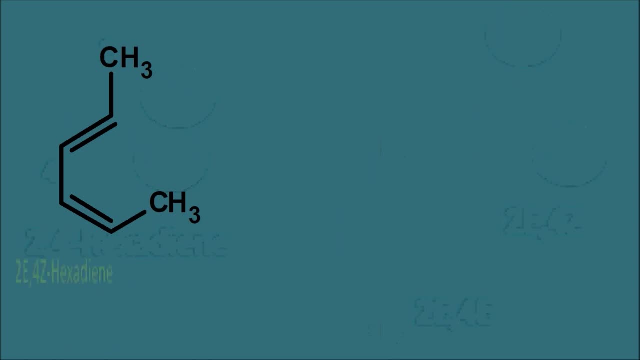 configuration. and let us see what happens to this electrocyclic reaction. now this is the 2e4z configuration or 2e4z hexadiene. so you can see the one of the methyl group is opposite and another methyl group is on the same side of the double bonds. now this compound can undergo the electrocyclic 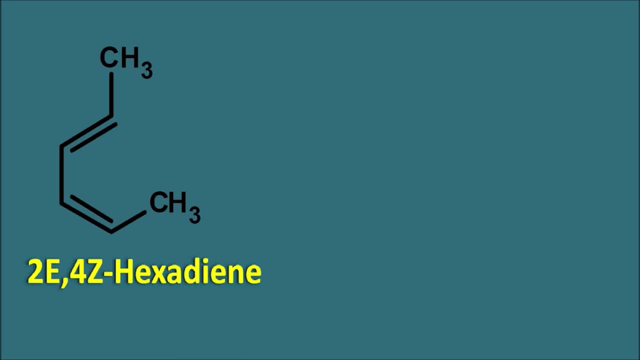 reaction, either by thermal source or the photosource. what happens when we use the thermal source? so, in presence of the thermal source, this compound can be converted such that it is going to give a product like this. now here, this methyl group and another methyl group on the similar side. so this is nothing but. 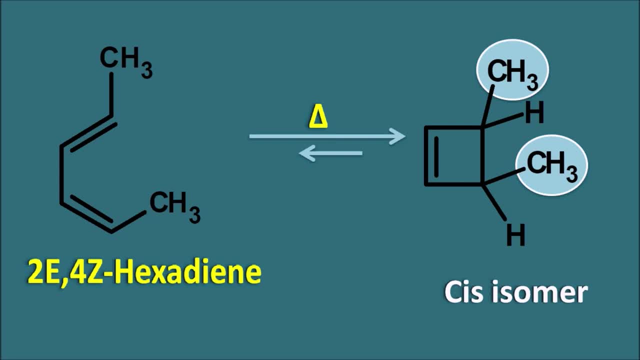 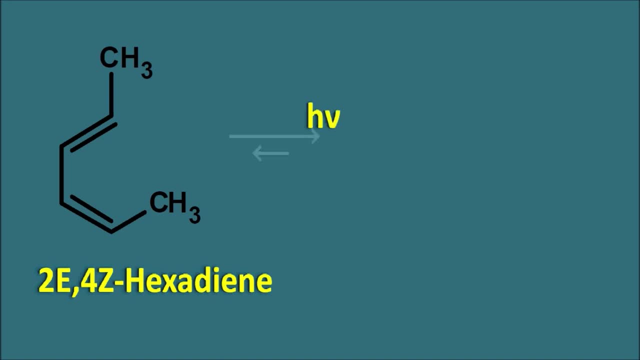 the cis isomer of the 3,4 dimethyl cyclobutene. now let us take the same compound, 2e4z hexadiene. but now we are going to use the photo energy. then what happens? the reactant will give one product. 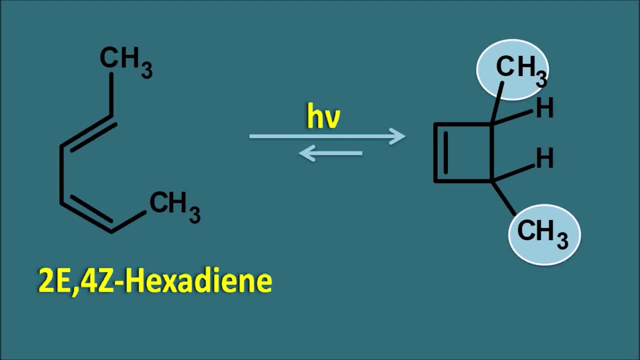 so here, one methyl group on one side and another methyl group on the other side. so this is the trans isomer. you can see here the same reactant. when we use the thermal energy, it gives the cis isomer. when we use the photo energy, it gives the 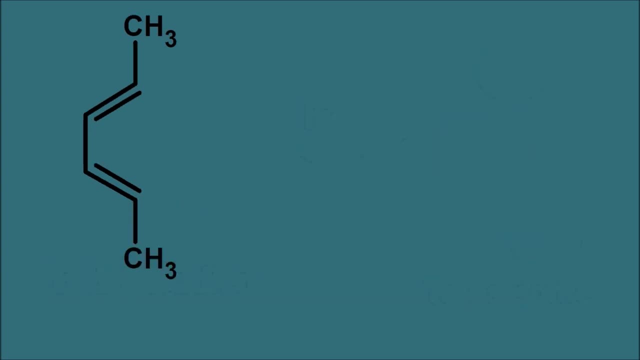 trans isomer. now let us take the another configuration. this is the 2e4e hexadiene, and when we supply the thermal energy, it is going to give a product like this here: the methyl group on one side and then the methyl group on the other side. so again, it is giving the trans isomer. 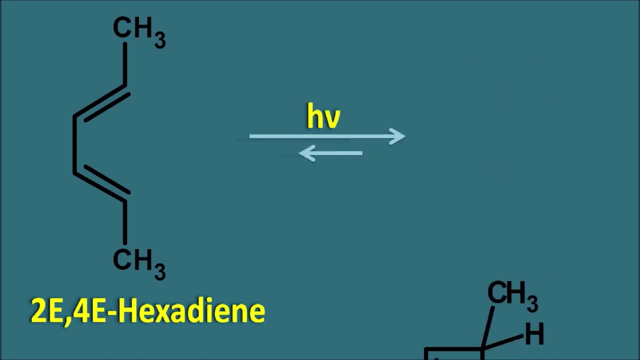 and to the same reactant. if we are going to supply the photo energy, then it is going to give a product with the cis configuration. the nature of the product depends on the source of energy we are going to supply as well as the configuration of the reactant. here we can summarize that: the 2e4z hexadiene on supply of thermal energy. it is going 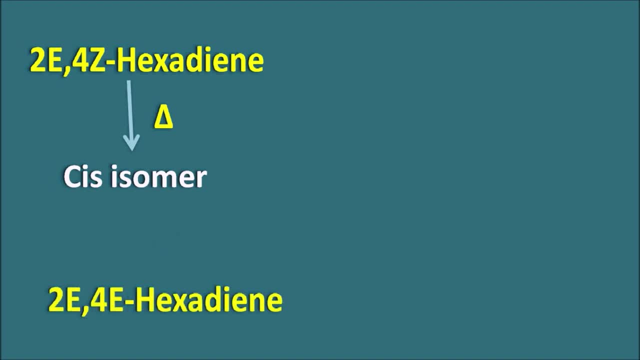 to give the cis isomer, on the other hand, 2e4e hexadiene, that is the ender isomer, having the different configuration, where at the fourth position it is having the e configuration and the photo energy. again, the source of energy is quite opposite. it is not the thermal energy, it is 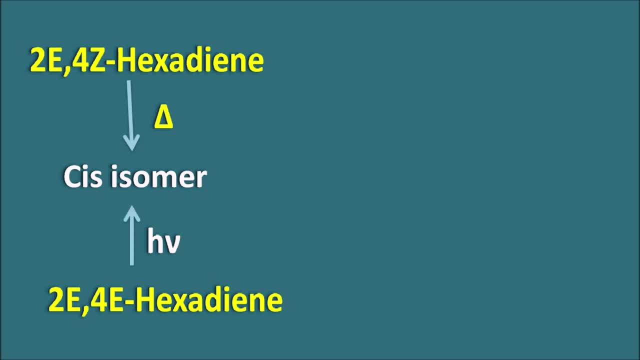 the photo energy, then it gives the cis isomer. similarly, the 2e4z hexadiene. when it is supplied with the photo energy, it gives the trans isomer. at the same time the 2e4e hexadiene. when we supply with the thermal energy, it gives the trans isomer. that means the 2e4z and 2e4e are going to produce. 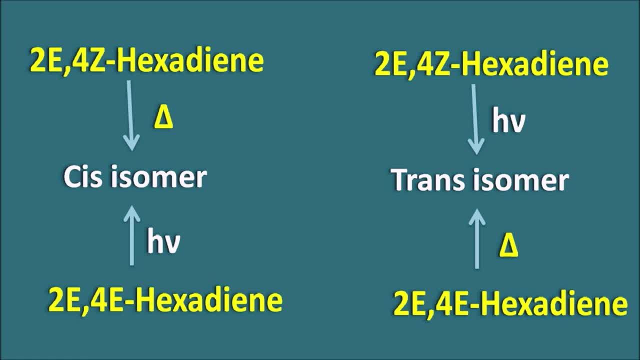 the same isomer when they are supplied with the different source of energy. so this is the trans isomer energy. one is thermal and another is a photo energy. right now it is somewhat confusing to remember, but we will see one of the trick by which we can easily remember the configuration of the 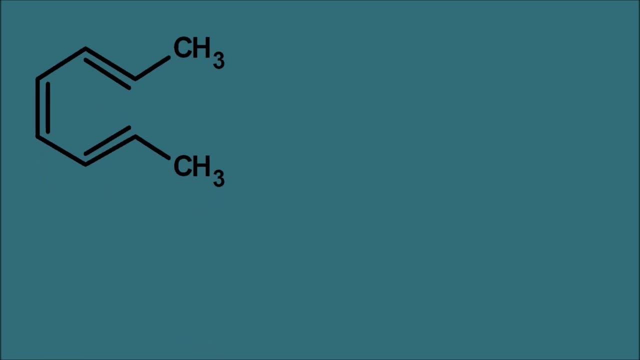 product. now let us take another example. so this is the reactant, this is the second carbon and this is the sixth carbon. and again, if we focus the methyl groups at the first double bond and the last double bond, they can exist as the different configuration. so this is one of the configuration. 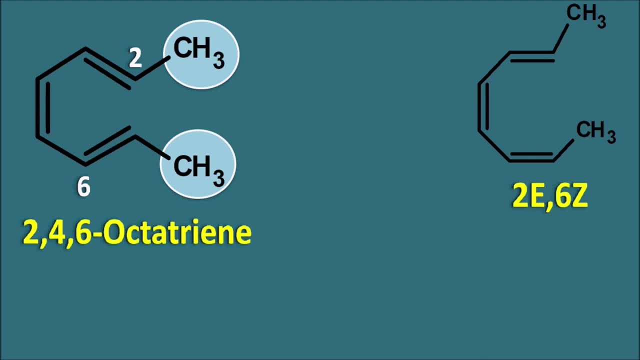 which is nothing but that 2e and 60. at the second position, opposite configuration, but at the sixth position, same configuration. Similarly, another one is the 2E6E, both at the second position as well as the sixth position. methyl groups are oriented opposite to the double bond. Now, with these two configurations, let us see. 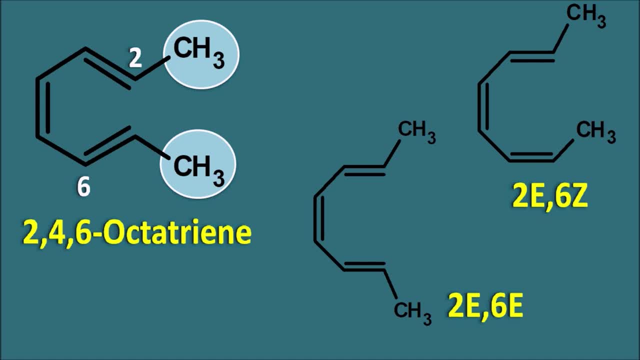 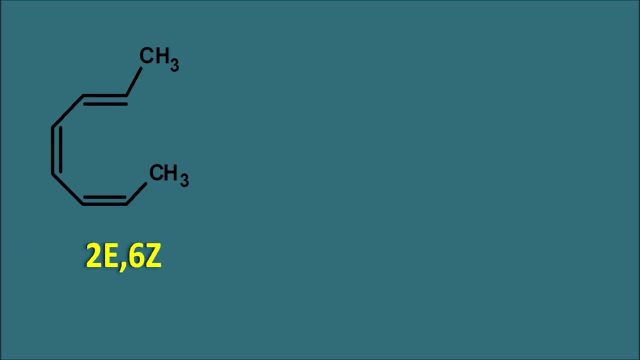 what happens to the configuration of the product. First of all, let us take the 2E6Z isomer. So this is a 2E6Z isomer here. we have not indicated the configuration of the double bond at the fourth position, for easy discussion Now, when we are going to supply the thermal energy it will undergo. 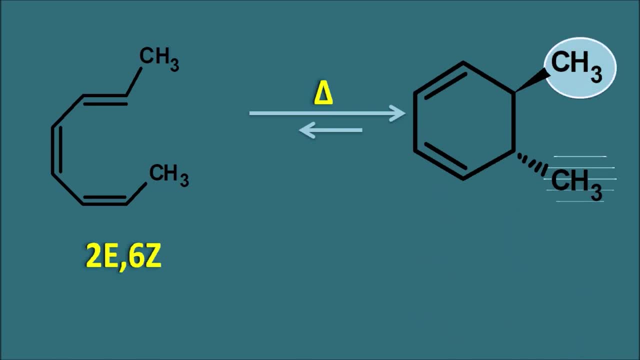 the reaction such that it is going to give a product like this. and here the methyl groups are in the opposite configuration. so these are trans isomer. So 2E6Z on thermal source gives the trans isomer. This is quite opposite with the previous example, which is having the two double bonds only. 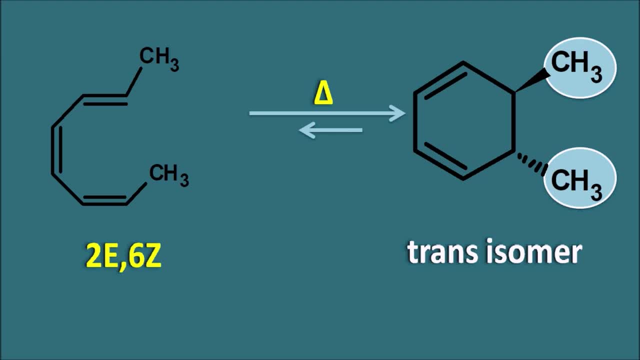 So when it is having the two double bonds, with 2E and 4Z configuration, it gives a cis isomer, but here it is not. It is going to give the trans isomer. Similarly, when it is going to react with the photo energy, 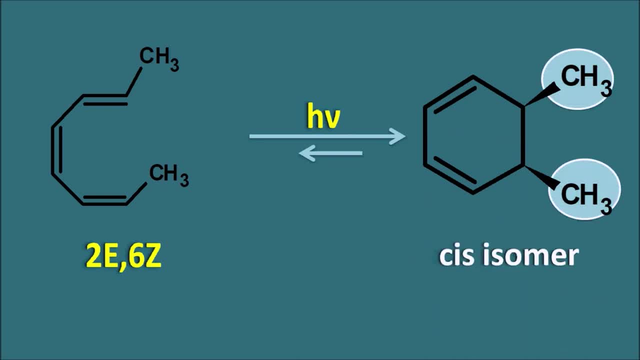 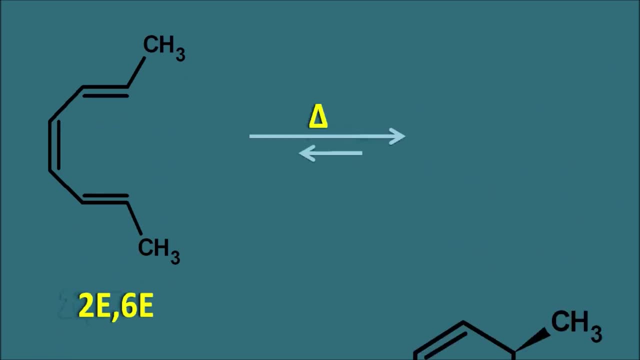 it gives one of the isomer here the methyl groups on the same side. so this is the cis isomer. Similarly, let us take the 2E6E. Now, when it is reacting with the thermal source, it is going to give the one of the product with methyl groups on the same side. this is the cis isomer and the same. 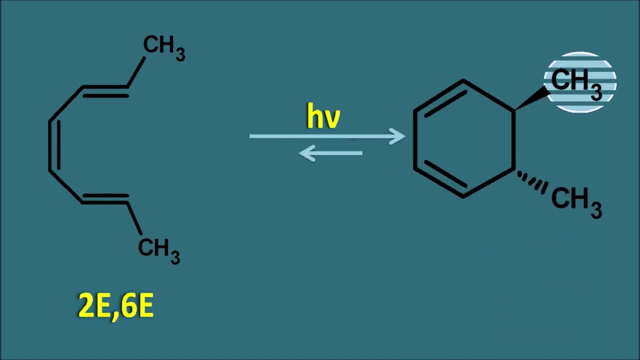 compound on the photo source. it is going to give the one of the product with methyl groups on the opposite side. so this is a trans isomer. In this way the compound with the three pi bonds is going to give the different types of products. Let us summarize it: 2E6Z- octatrain on supply of thermal. 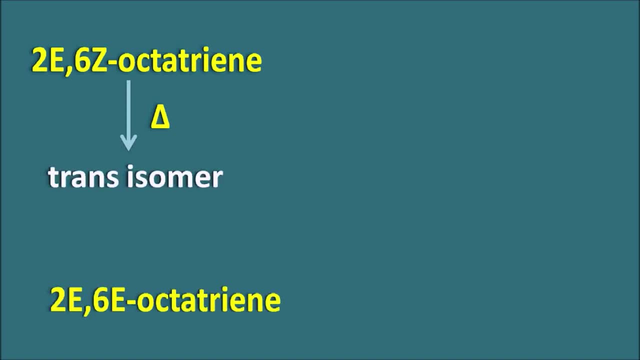 energy. it gives that trans isomer. Similarly the 2E6E octatrain on photo energy. it gives the trans isomer, 2E6Z octatrain on photo source. it gives a cis isomer and 2E6E octatrain on thermal energy. 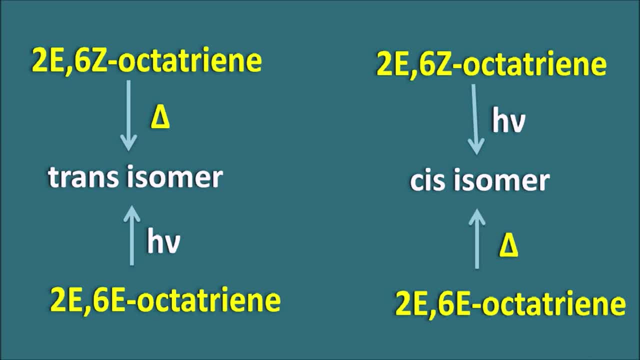 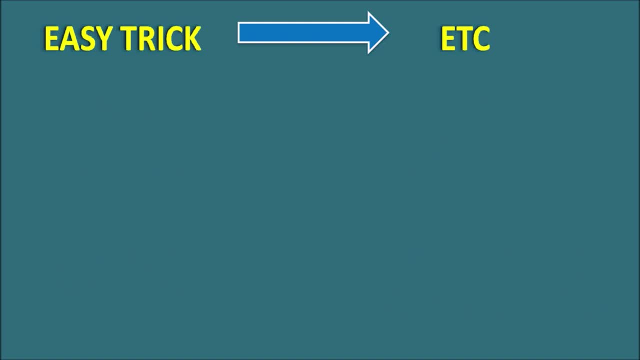 it gives a cis isomer. Some logic is there, we can easily remember. So now let us see the easy trick to remember this configuration. So here ETC means, E indicates even T, thermal, and C is the cis isomer. Even thermal cis isomer, we can easily remember. So suppose here we are going to take the 2E4Z. 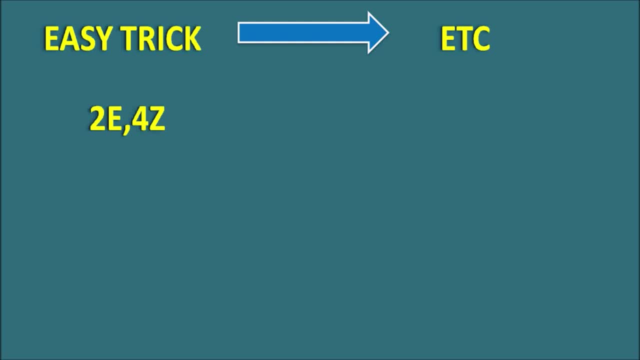 So here, 2E4Z means: how many double bonds are there? only two double bonds are there. that means it's a even so even number of pi bonds are there. and what about the configuration of these double bonds within the reactant? one is E and second one is Z. that means within the 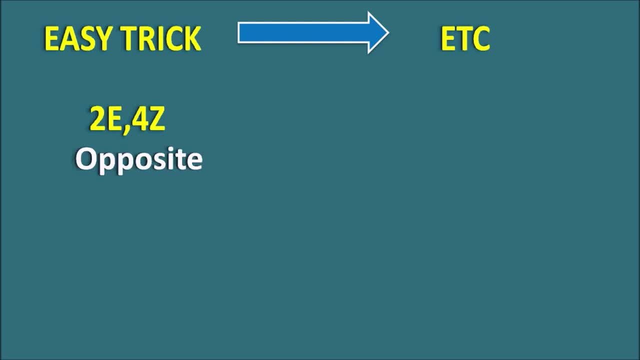 reactant, it is having the opposite configuration. Then when we supply the thermal energy, it will give the product with cis isomer. So here we can just remember with the trick: ETC, ET, even and thermal. let us take the this combination as negative. and what about the configuration of the reactant is? 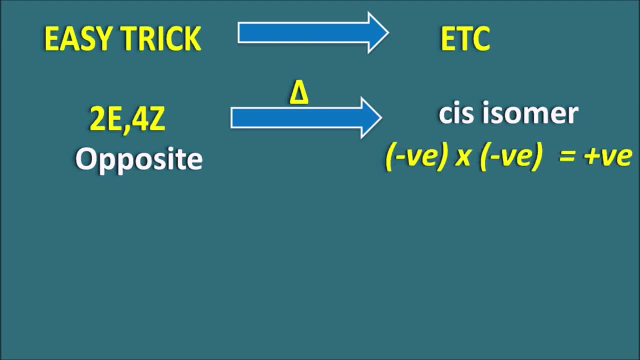 opposite. Opposite means again negative, So negative into negative will give the positive, So positive means they are the cis isomer. Similarly, if it is not, even if it suppose, if it is odd, let us take one example: 2E4Z6Z. Now here it is, having 3 double bonds. 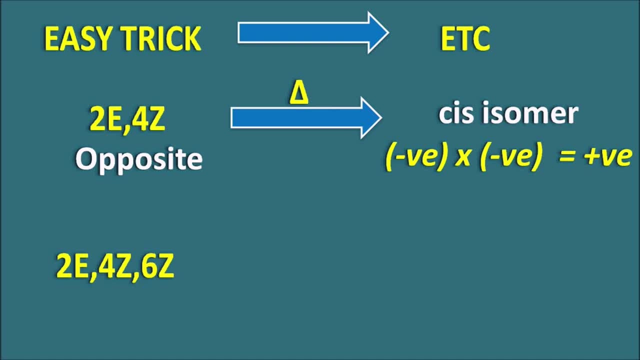 so it is having the odd number of pi bonds and if we see the configuration at the terminals 2E and 6Z, they are having the opposite configuration. Suppose we are going to use the same sub energy, thermal energy- then which type of isomer it will give? it will give the trans isomer. 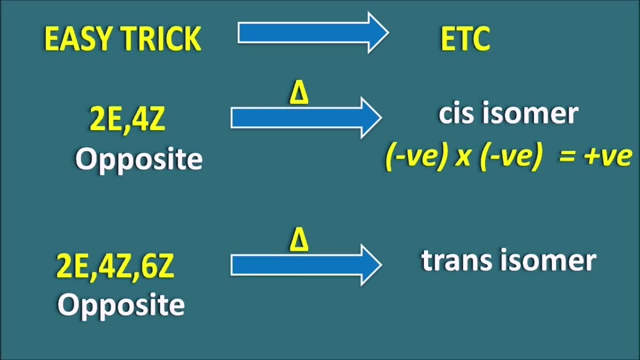 So here one of the condition is going to be changed within this combination. Even there in the Halen thermal the even is replaced with the odd, then the product will have opposite configuration. So when it is odd it will be negative into positive, which gives the negative So opposite. 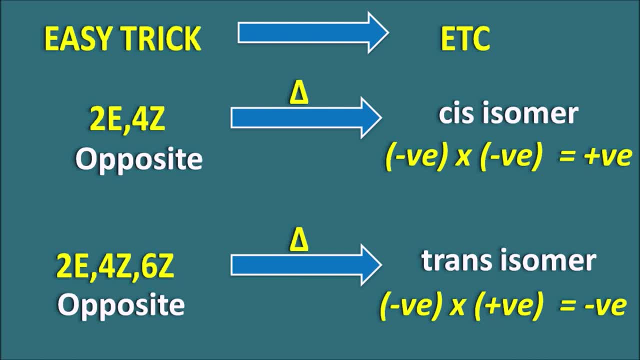 configuration can be upset In this way: if even is replaced with the odd, it will give the opposite configuration. Otherwise, if the thermal is replaced by photo, it will give the opposite configuration. Otherwise, if the reactant is having similar configuration, again it gives the opposite configuration. In this way, if any of the condition is going to be,